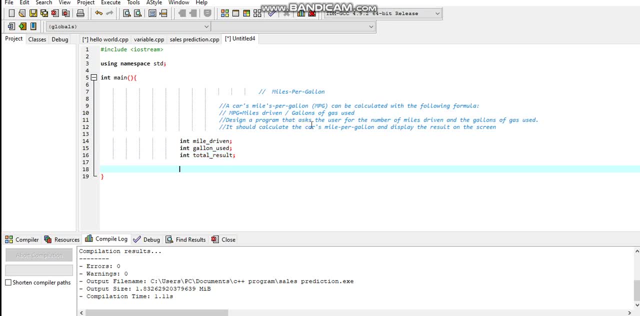 so, first of all, what we're, what we're told, is that design, we should design a program that asks the user for the number of miles driven, so, which we can we are going to do right here: c out: please enter the number of miles driven. please enter the number of miles driven by any number given to it. 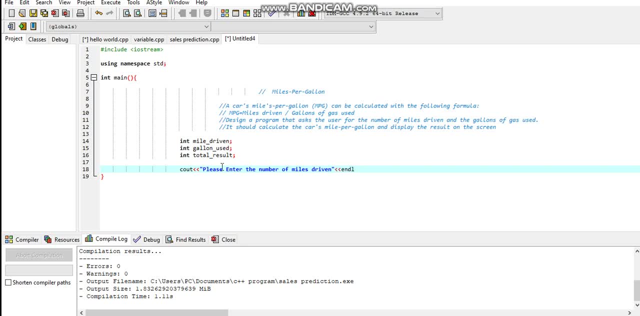 we are going to install it somewhere, end line, we're going to see in, and then i please, i will continue to say, take note of these errors. the point in this one is pointing this side, uh, on your left, and this one is pointing on your, on your right, when you are storing something on a variable. so please enter number. 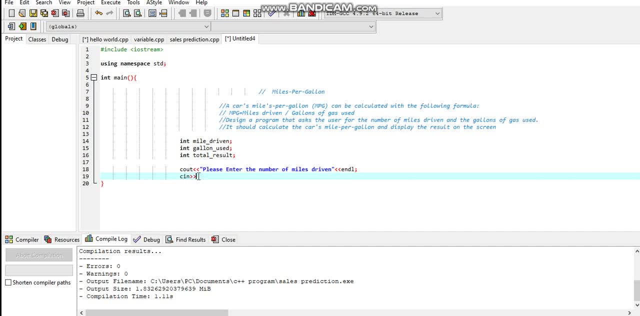 of miles driven where we're going to spot, uh, install it, or why we're going to store some, uh, what the person is going to drive, then we are going to don't look for it. so inside i'm going hold something, i'm going to reserve a model, ah, select other variables to speak for. let me do that, just uh. 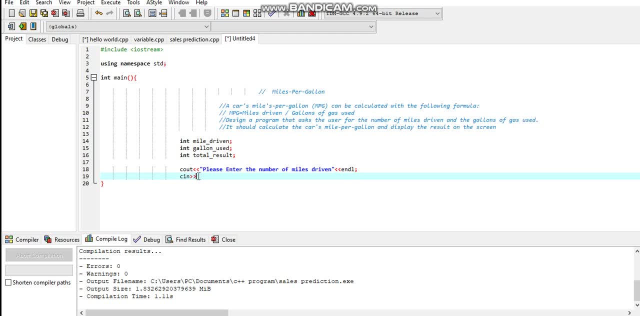 to enter. if the person enter my driven, so we're going to store it on the mine driven variable. and then what are we what? we're also told that we should allow the user to enter the gallons of gas used. so we're going to say c out again. um, see out, please enter the gallon. 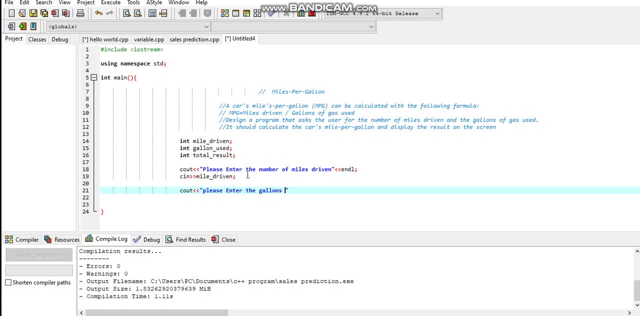 okay, is that colon used? how many gallon, what, where? where did you use this this month? so i'm gonna end that line right now and i'm going to store it somewhere called so in the variable code card. so i'm going to store it somewhere called so in the variable code card. 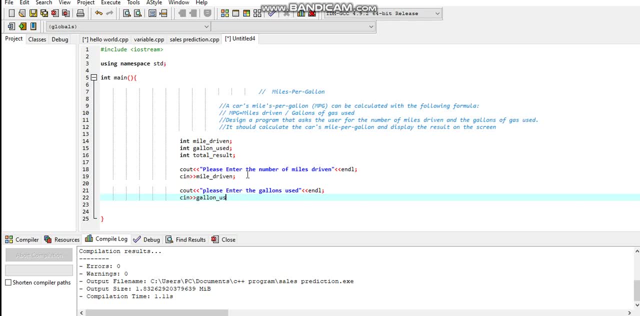 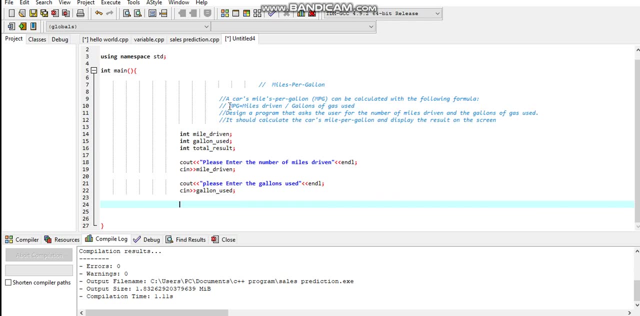 on gallon, um used. and then we're going to: what do i? what did we told? we're told that, um, this is the formula we're supposed to use: miles. mpg is equal to miles driven. okay, so let's just say mpg. let's just don't put a result, let's just make it a bit nicely. let's say mpg, right. mpg- miles per gallon. 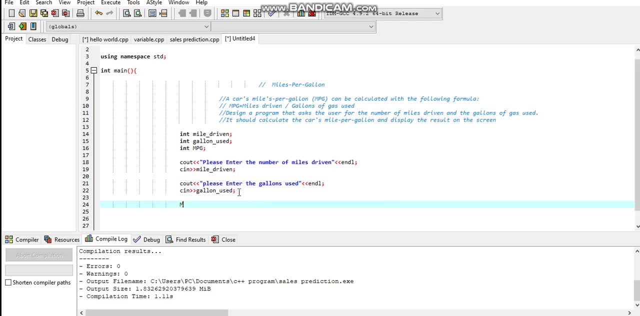 right. so we're told that mpg. now we are assigning the value mpg. shouldn't we just assign it right here? okay, yeah, let's just assign it right here. so mpg is equal to miles driven, which is my, our variable. my driven divide by what a gallon use, gallon um used, that is the variable. 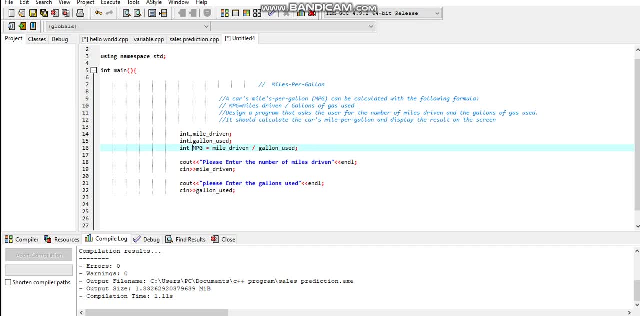 so this one, this mpg minus per gallon, is going to contain this one, the, the. after the computer divide the program, divide this one it would. this is what to do. it will divide these two and assign the result into this variable, the mpg variable. so we're going to 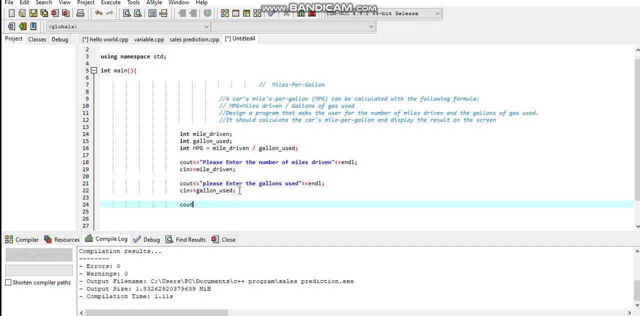 print it out on the, on the screen. see out, oh dear, let's just make it a bit nicely. oh yeah, you just how do you spend that again? you just, um, did the best calculation ever. does that make sense, even if, anyway, that's just something kind of dumb. 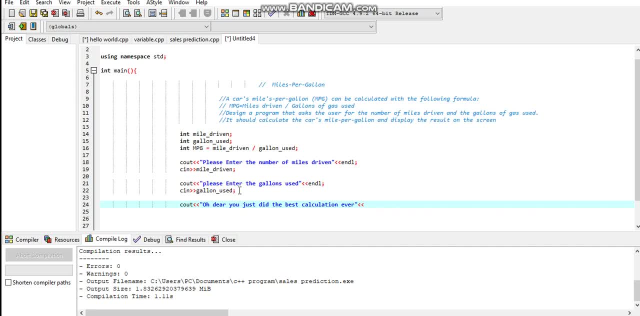 but fine, all right, um, let's just print it out and that's the um, mpg, mpg, mpg and the list end line, right end that line. and then, oh yeah, you just did the best calculation ever. let's just put some space here. okay, you can also put it. it's possible to take this thing and put it on on the underneath. 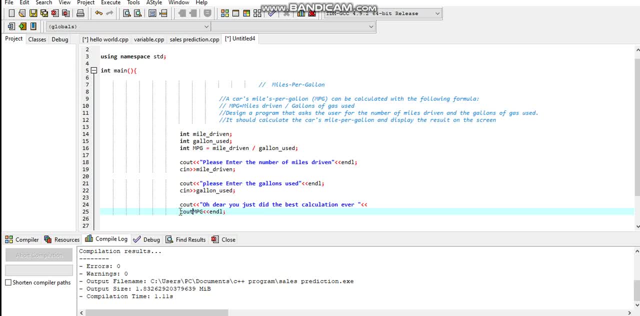 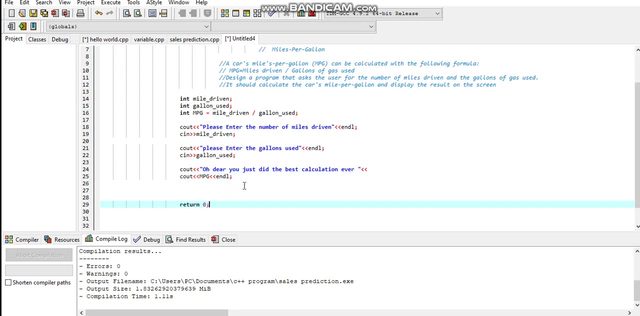 it's still okay, you can just say c out again, but i like putting it on the, on the. i mean, yeah, on the same line. so let's just run that. should i return it by zero, because our program will run successfully, obviously, but we wanna, we don't know, let's. 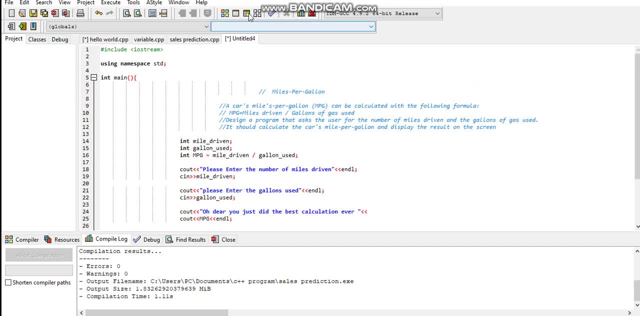 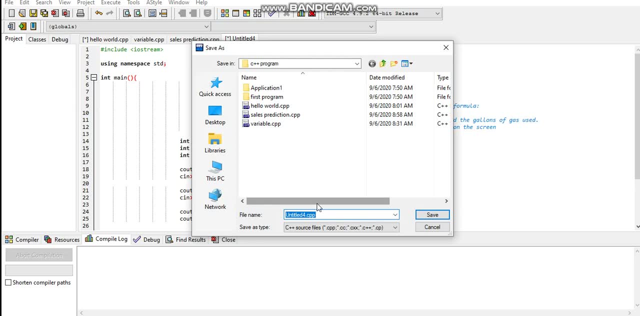 make computer understand. and then we have done writing our program list computer. let allow computer to do his own thing. so let's compare, compile it and then let's save it as um. i like saving it the title of our program and then mpg, miles per gallon. okay, i don't like spelling, i don't know. i'm flopping, which is with writing things. 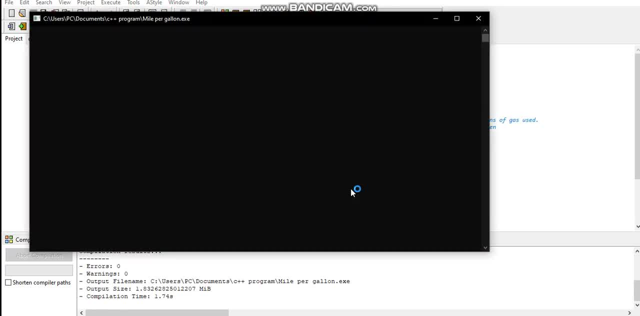 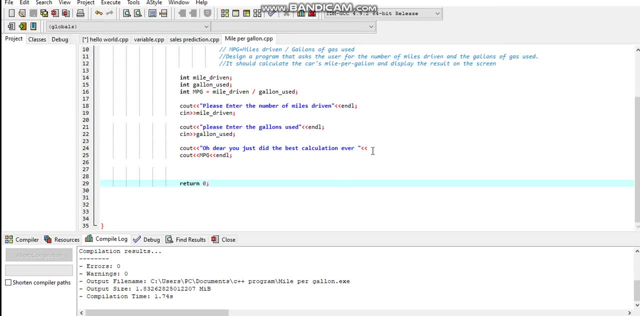 but i'm gonna just gonna do that. there's something i'm. i made a mistake somewhere, but this computer did not recognize that mistake. why is it writing? writing this? okay, let's just see what the mistake that i wrote. i wrote this, i didn't terminate, but still it. it is still um printed out. i must. 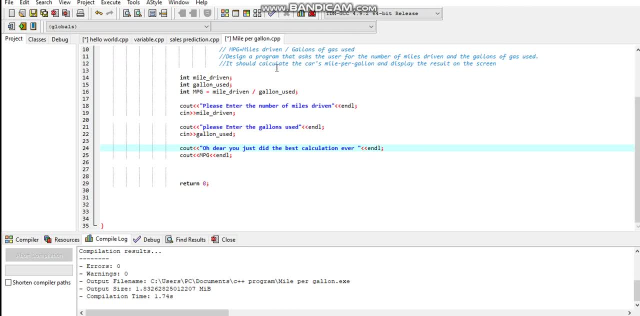 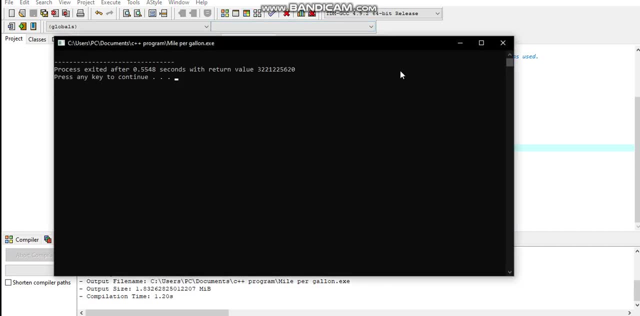 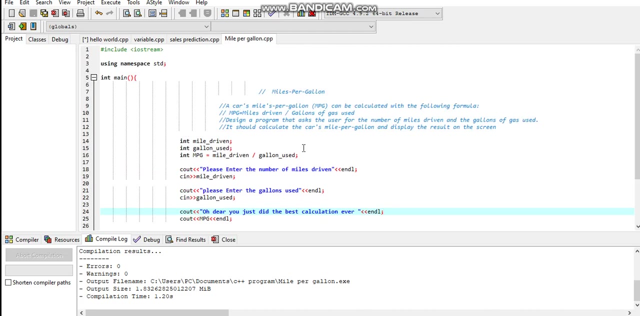 terminate end line and then let's um run it. oh now, okay, i think that i'm gonna fix this error right now, because i really don't know why it's not displaying the thing we wanted to display. so i'm just gonna close this thing off. i'm just gonna close this thing and then 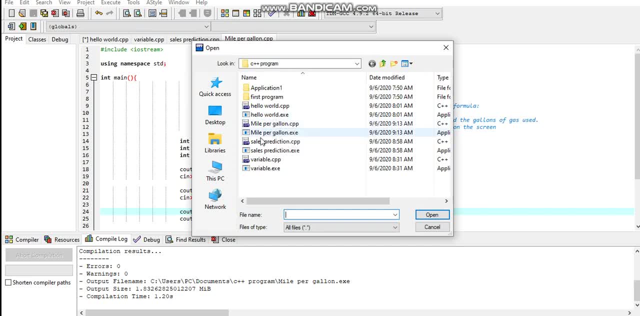 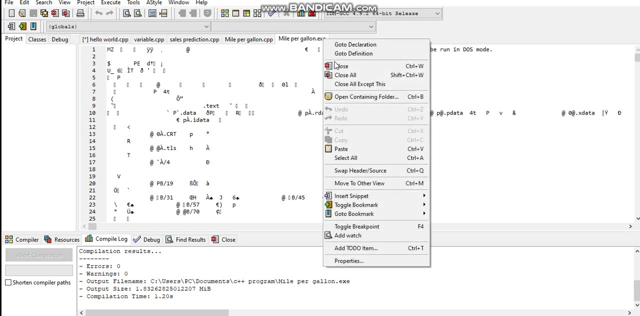 open that. maybe i should just open it. and then, um, of course, when you, whenever you write, you have the source file and then you also have the extension file, executable file. it's nice, so let's just click on it. whoa, oh, let mama. this is just so nice. 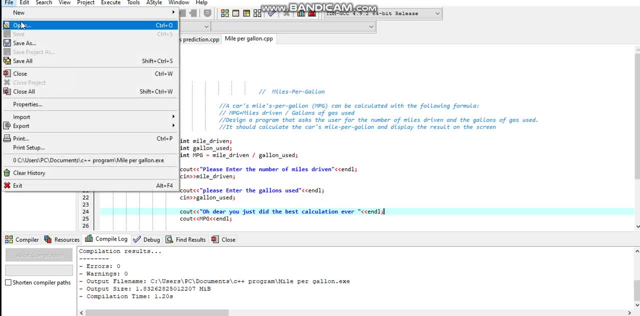 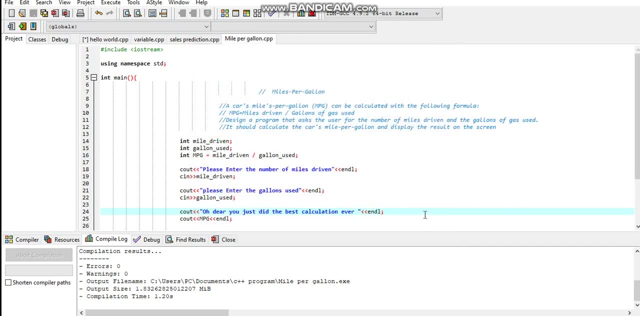 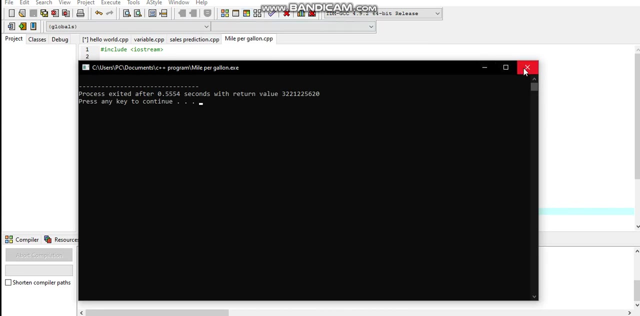 okay, so let me just open that again. i really don't know what happened just now, because this computer just messed up. i think it's because i've been using it to let me just see. okay, let me just run it. program is it? can this be true? where is my wrong doing? lucky, lucky, lucky, lucky, lucky, lucky, lucky. 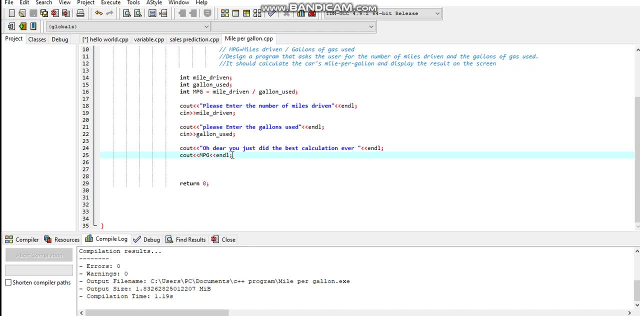 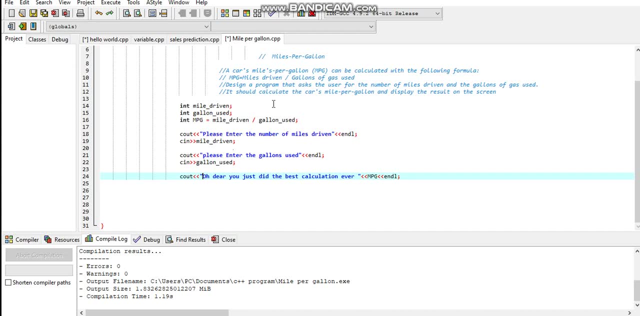 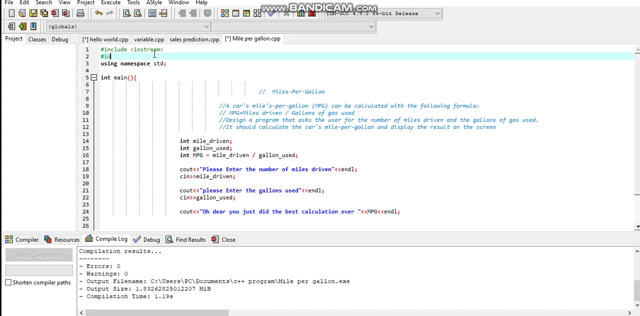 let's just, uh, okay, i don't, i don't know, let me just put it back here, and then let's see what we've got my driven. it mean, okay, let's just say string, hashtag, include, include, string, okay. and then let's just, um, okay, i don't know, but okay, just give me a minute, and then let me just the do this, just so fast i 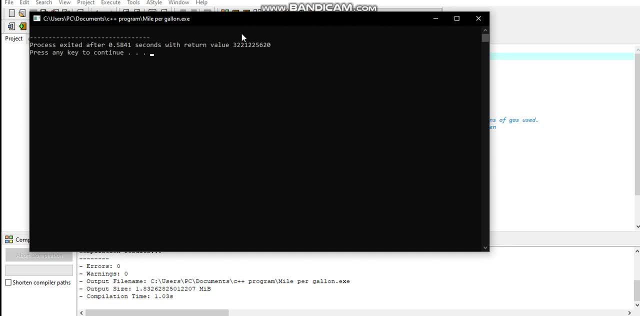 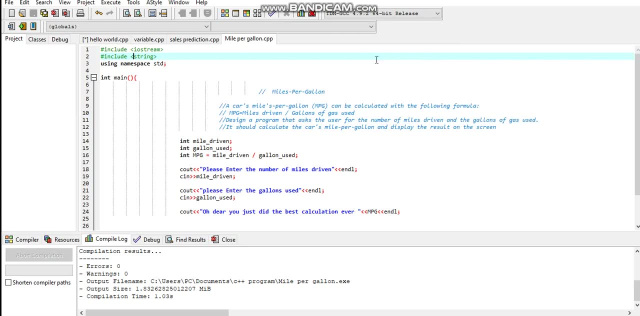 doing right now because i i think i designed this in really cool. and then now, okay, you know what guys? um, thank you for watching my tutorial. i'm gonna sort this thing out and i'm gonna give you the, the, the why, the why, what, the reason why we can't start this thing. but i think in the next,